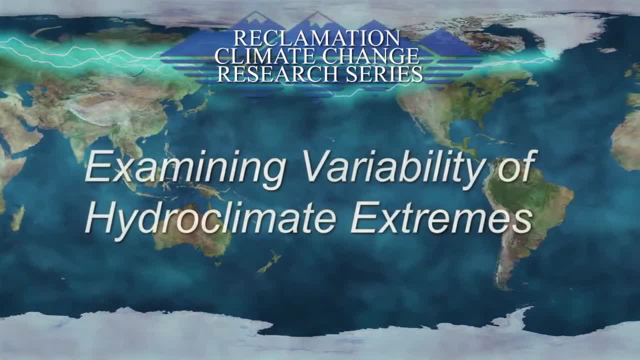 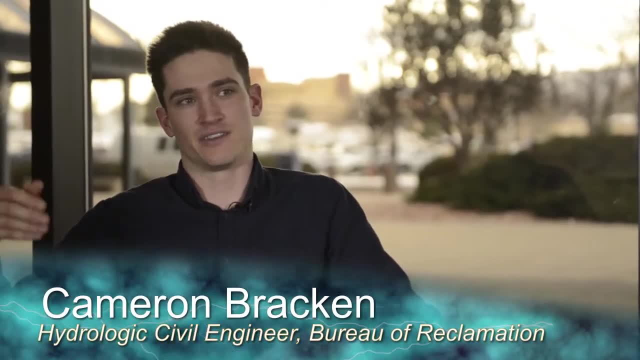 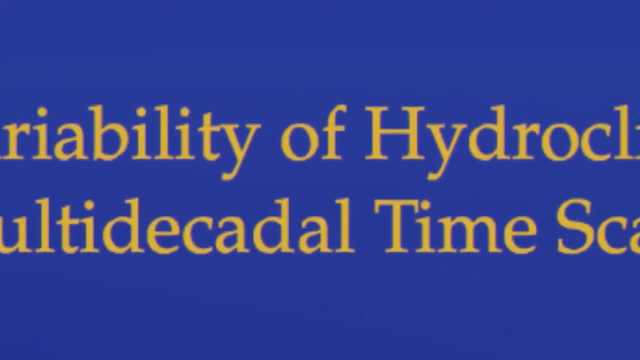 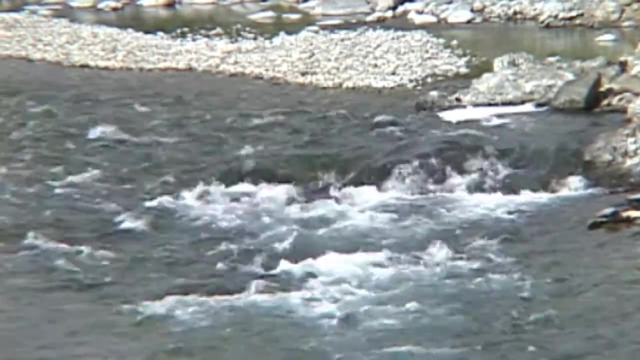 Yes, we need to stay abreast of the modern research and incorporate that into the work that Reclamation is doing. I'm looking at the variability of hydroclimate extremes, which are both streamflow and precipitation in the western US. so Reclamation's region. 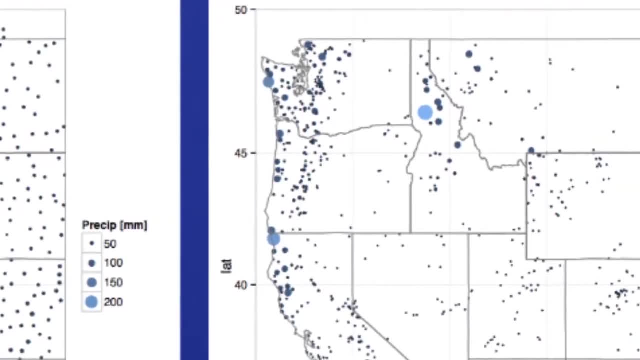 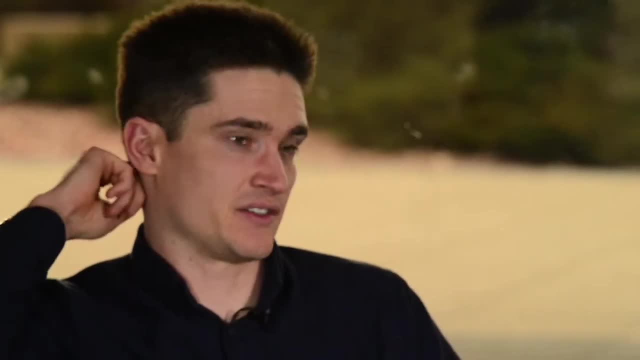 of interest and looking at how the extreme events vary spatially and temporally. We're looking at patterns of behaviors over multiple seasons or within one season, or multiple years, and we're looking at how those things change from year to year and, hopefully, how they change. 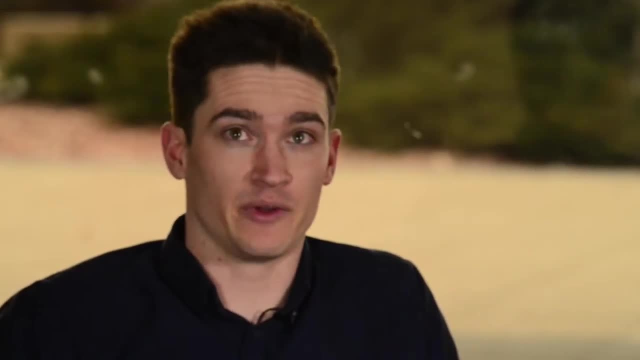 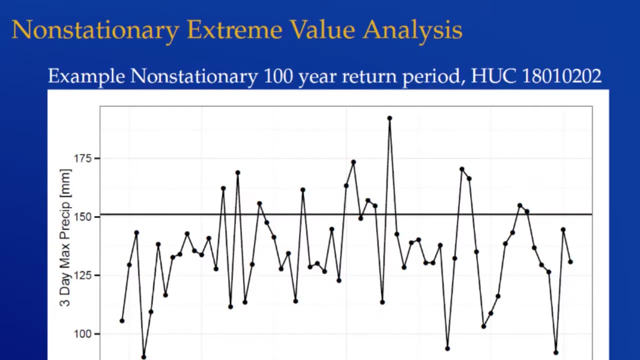 into the future. It might take the form of like: alright, we think over the next 10 years, the highest extreme event you're going to see is going to increase by 20%. That might be the type of event that we're going to see. 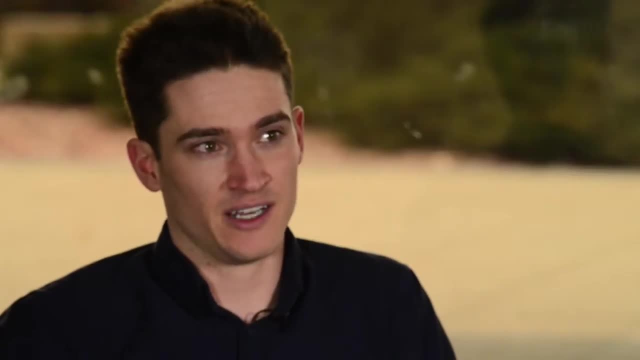 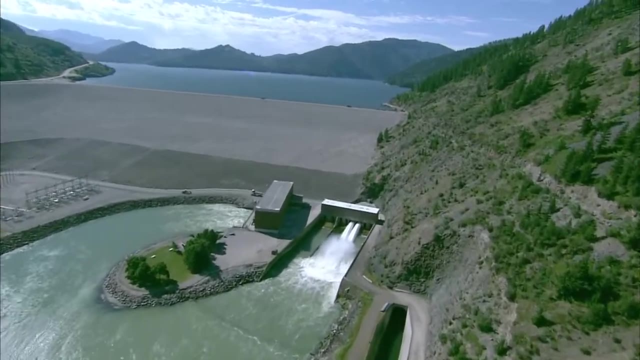 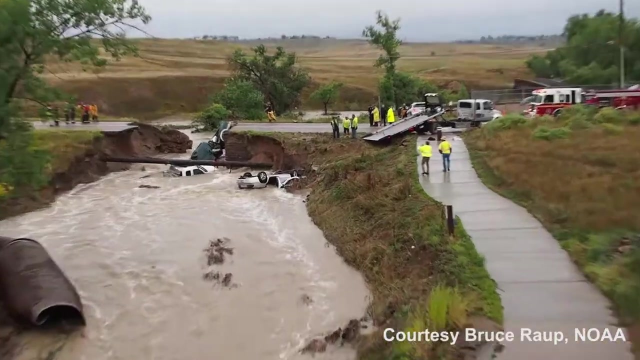 So it's not just the information that they're getting, but still that's incredibly useful to know if that's going to be increasing, staying the same, decreasing. The goal is eventually to look at impacts for infrastructure planning into the future. So if extreme flooding events are going to get larger in the future, we want to know. 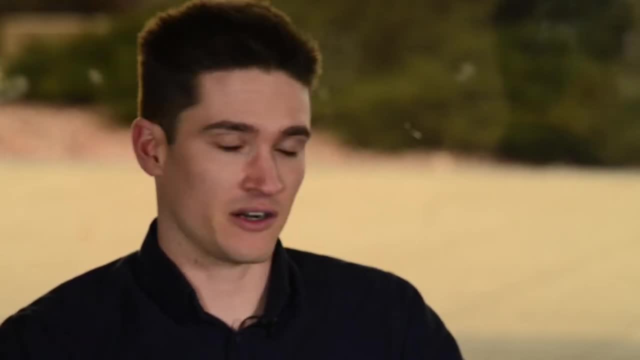 that that affects how we manage our reservoirs. If they're going to get lower, we also want to know that that affects how we manage our reservoirs. Yeah, one of our tasks that we're doing right now is managing the reservoirs, So one of 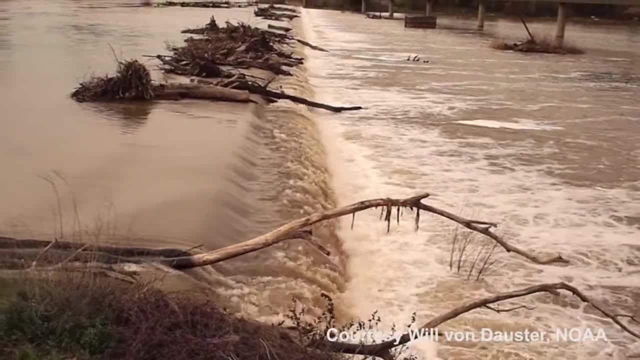 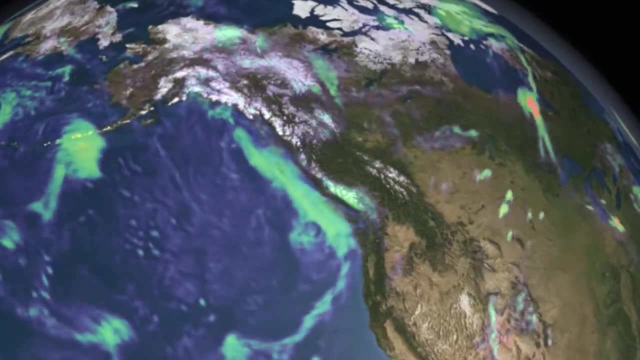 our tasks that we're doing now is managing the reservoirs, and one of our tasks that down the line is to develop some sort of tool for water managers. The ultimate goal is to provide sort of a map that you can look at for any place in. 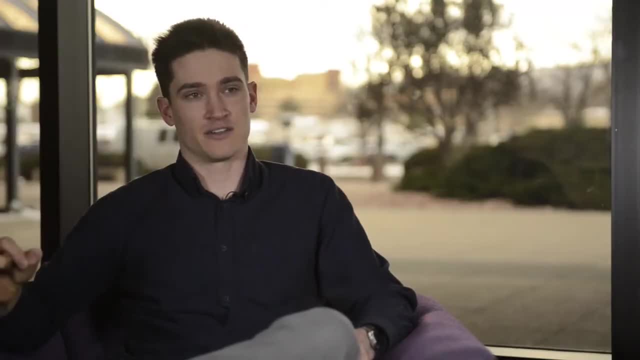 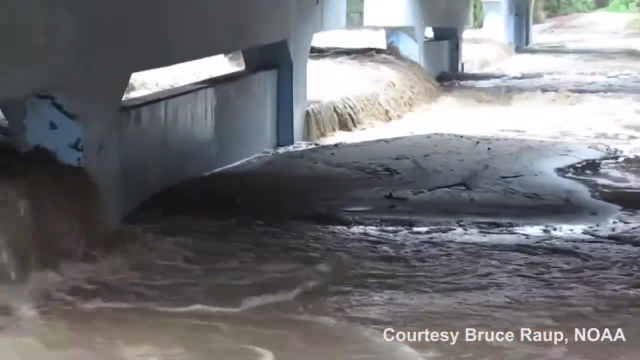 the western US and say, okay, this is how hydroclimatic streams are going to change here versus here, versus here, Like the precip generates the stream flow and you can't look at these things separately. You have to look at them together to get a complete picture. 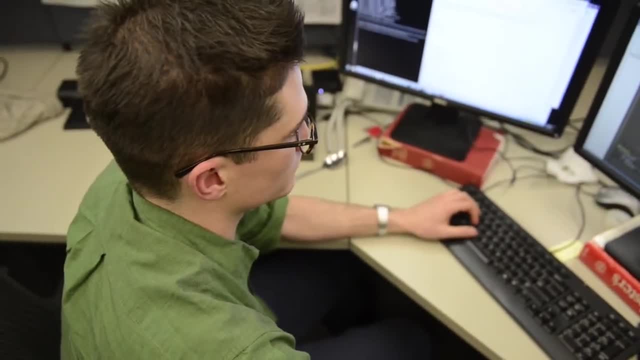 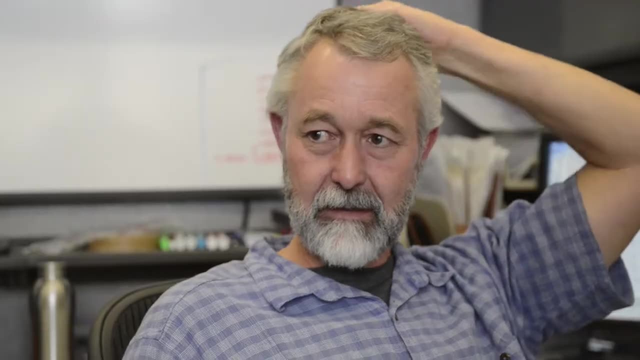 Reclamation funds all this research, including mine, that is all based around. how is this going to be used to be helpful for humans? Here at Reclamation we're like it sounds cheesy, but I feel like I'm doing the right thing.